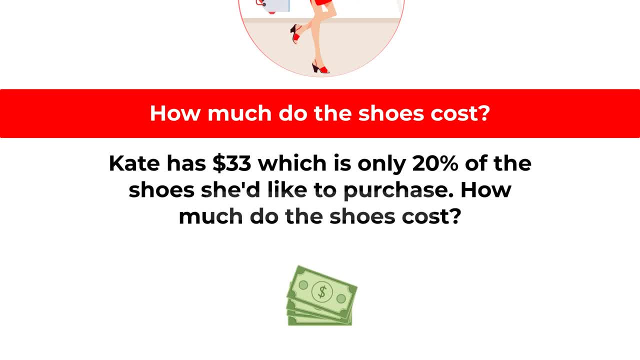 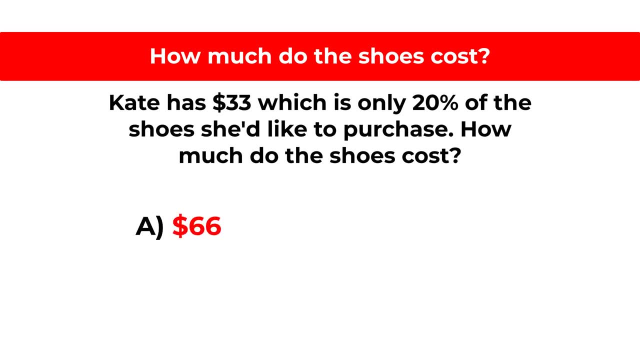 the cost of shoes that she would like to purchase. How much do the shoes cost? And you're presented with four different choices: Choice A: $66.. Choice B: $99.. Choice C: $1,000.. Choice C: $1,000.. Choice. $1,000.. Choice B: $1,000.. Choice C: $1,000.. Choice C: $1,000.. Choice C: $1,000.. Choice B: $1,000.. And you're presented with four different choices: Choice A: $66.. Choice B: $99.. Choice C: $1,000.. Choice C: $1,000.. 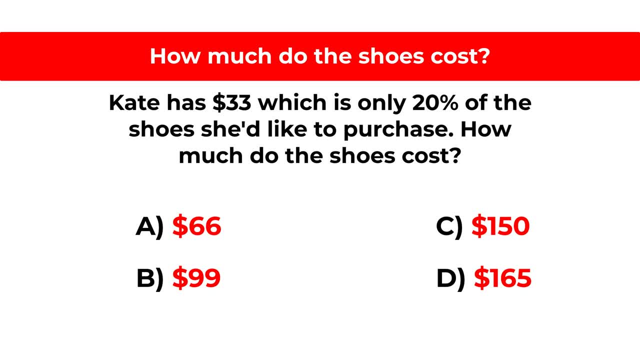 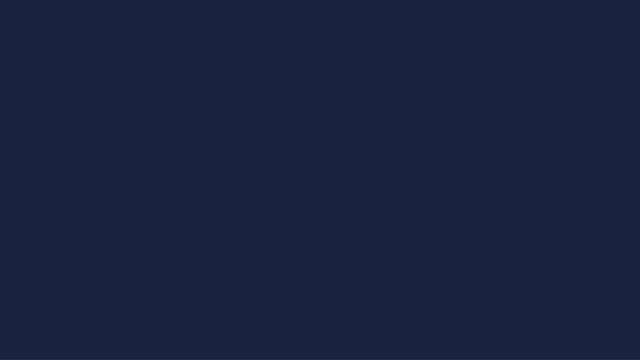 dollars and choice d: 165 dollars. can you calculate the answer? give yourself 10 to 15 seconds, maybe 20 to 30 seconds, depending how well you are with math and percentages, ready or not. let's go ahead and get to the correct solution together. the answer to this problem is very simple: 33 is 20 percent. 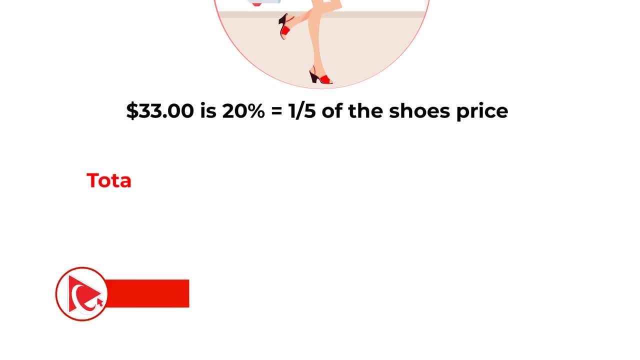 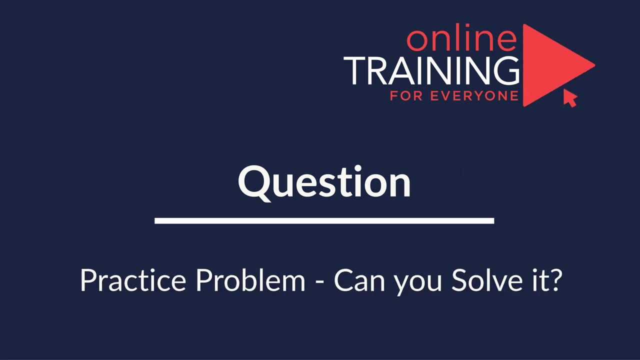 or one-fifth of the shoes price. so the total cost of the shoes would be 33 multiplied by 5, which would be equal 165 dollars. so the correct answer here is choice d, 165 dollars. and here is the practice question for you. you're presented. 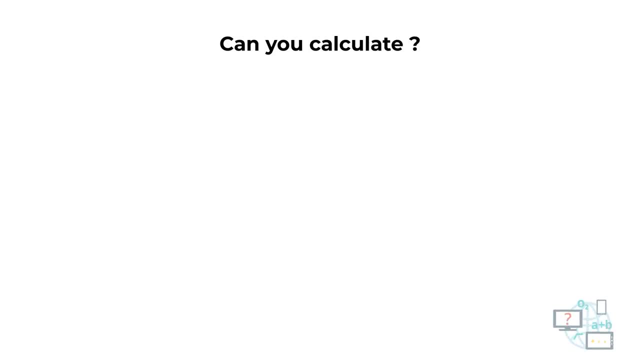 with three full expressions and you need to calculate missing number in the force expression. here are three full expressions: 18 by 3 equals 27, 12 by 4 equals 12, 22 by 8 equals 32 and you need to calculate the result of 12 multiplied by. 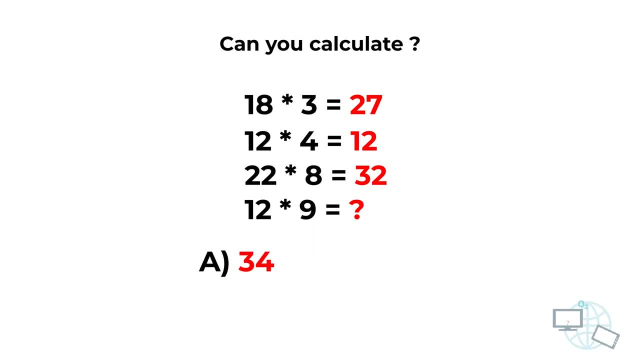 9. you have four different choices: choice a- 34, choice b- 36, choice c- 38 and choice d- 40.. do you see the answer? give yourself a little bit of time because the answer may not be obvious. i'm going to give you a quick hint. do you know why? it's always two digit number multiplied by one digit number. 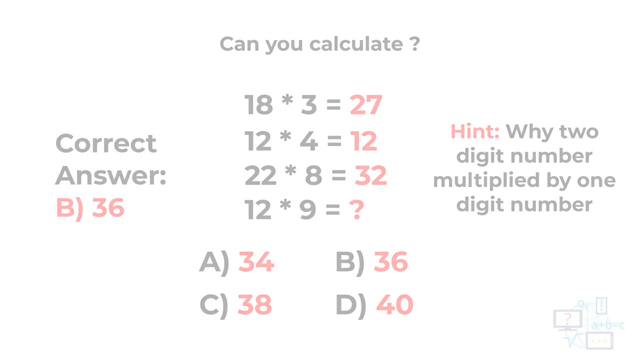 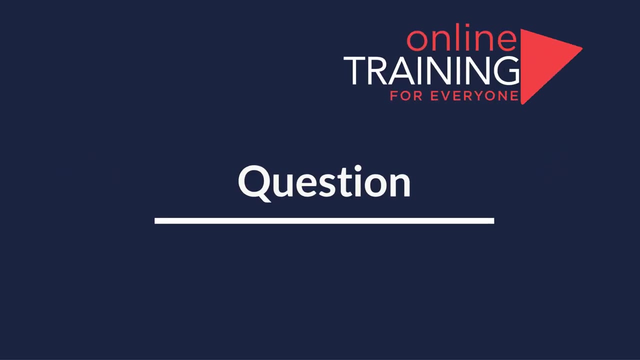 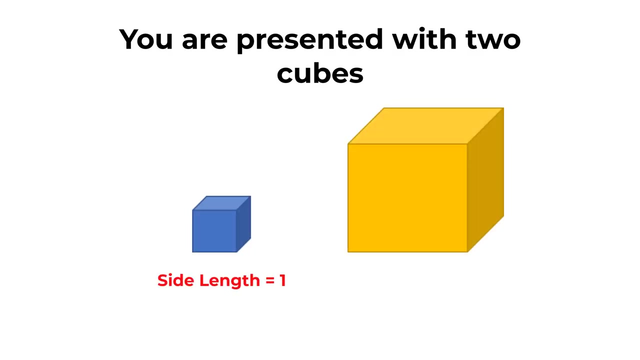 the correct answer here is choice b 36.. if you figured it out, please make sure to post your solution in comments. here's a cool question which you frequently see on the test. you're presented with two cubes. one cube has side length equal one unit and second cube 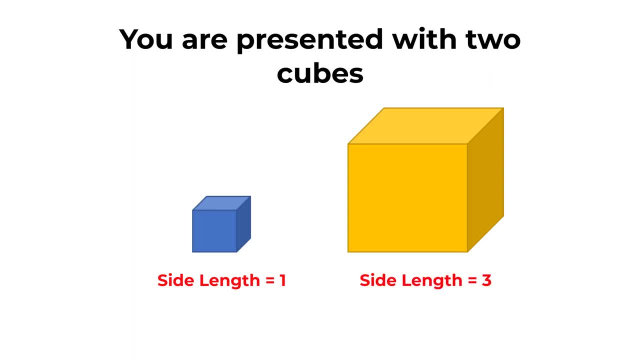 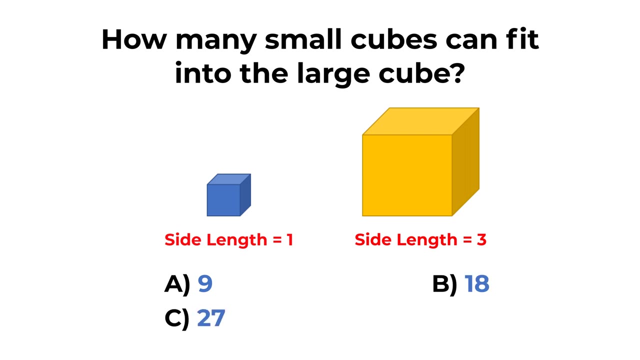 is a larger cube and it has side length equals three units. so the question is how many small cubes can fit into the large cube? and you have four different choices: choice a- 9, choice b 18, choice c- 27 and choice d- 81.. do you know the answer? give yourself. 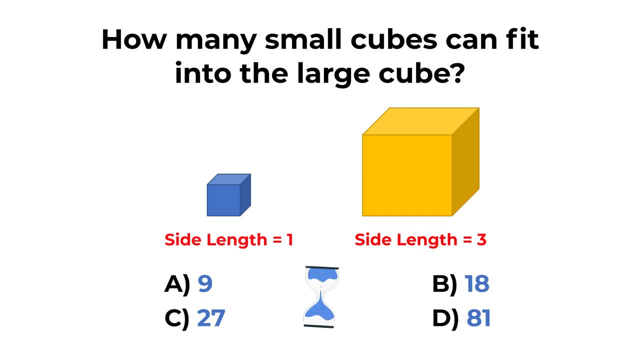 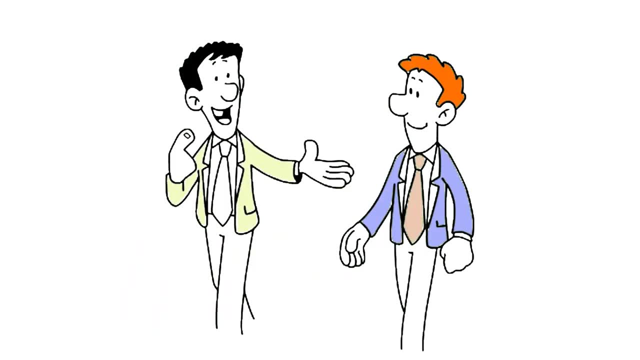 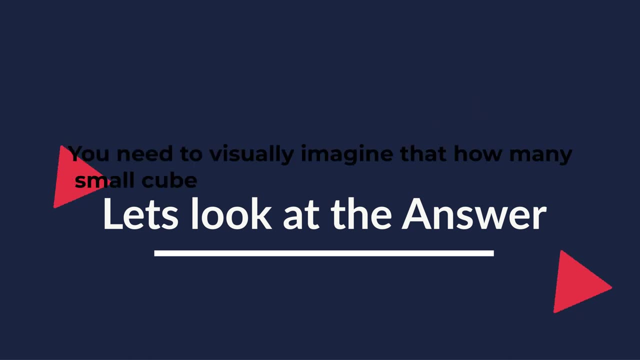 a few moments to calculate it, maybe 20 to 30 seconds. this is about as much time as you get in the real test, ready or not. let's go ahead and get to the correct solution together. to solve this. you can figure out how many small cubes can fit into one of the larger cubes. 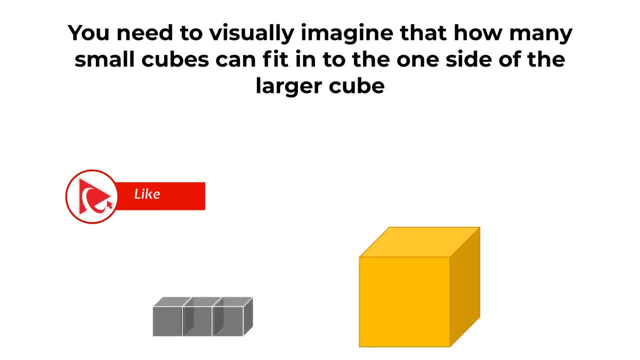 and the answer is that three small cubes can fit on each side of the larger cube. and since cube is three-dimensional, the number of small cubes that can fit into the large cube can be calculated using the formula three multiplied by three. multiplied by three, which is equal three. 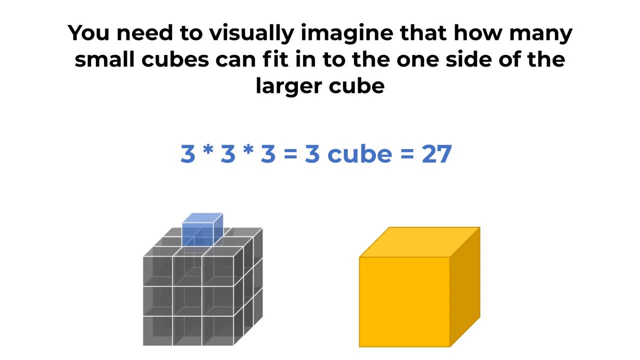 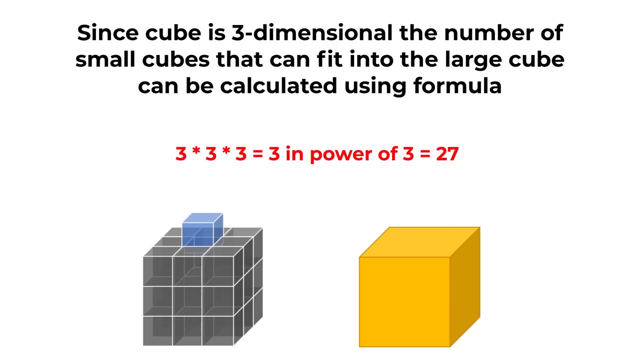 cube- that's where the word cube might be coming from- which equals three by two, so you need to equals 27.. Since cube is three-dimensional, the number of small cubes that can fit into the large cube can be calculated using the formula 3 x 3 x 3 equals 3, cube equals 27.. 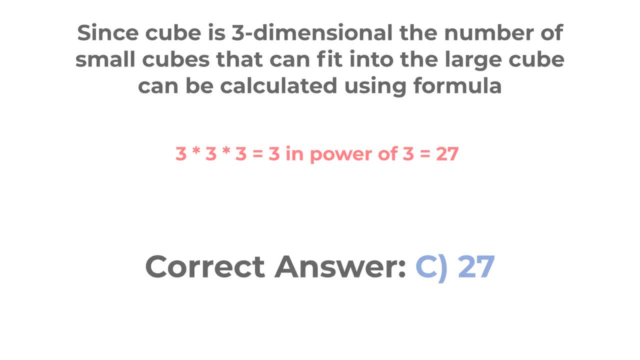 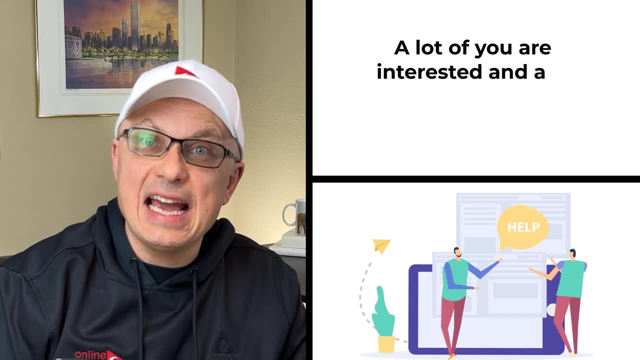 So the correct choice here is choice C 27.. Hopefully you've nailed this question and now know how to answer similar problems on the test. A lot of you are interested and ask me: how can I help others? One of the ways you can: 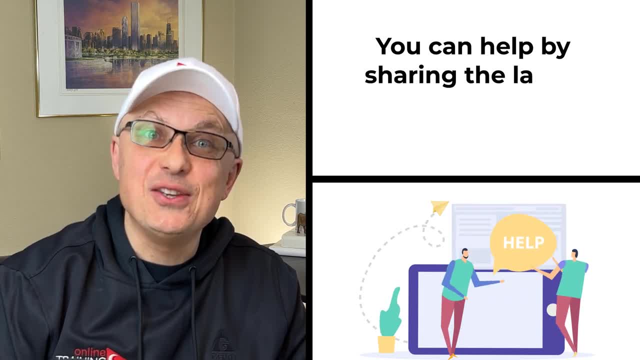 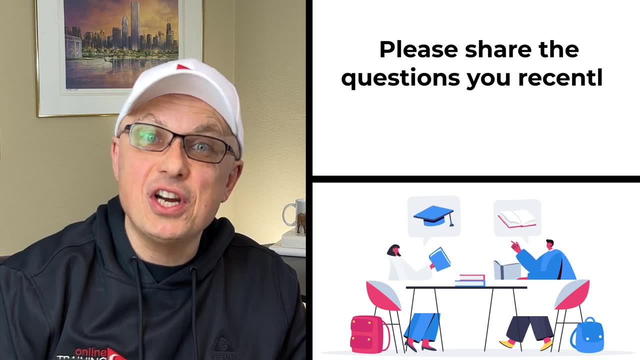 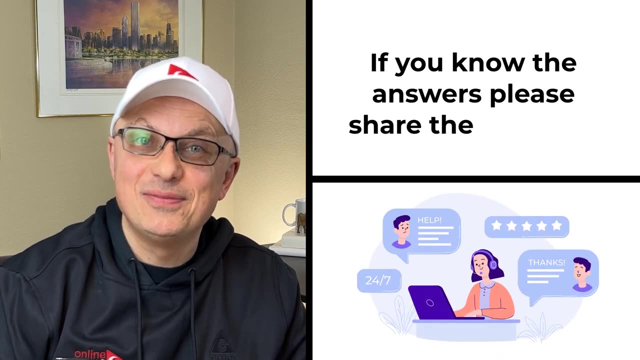 help other people is by sharing the latest questions you see as part of the assessment test, And when you share, please make sure to also include how you answered them. Please share the question you recently encountered in the comment section of this video And if you know the answers, please share them as well. And now let's continue and get you. 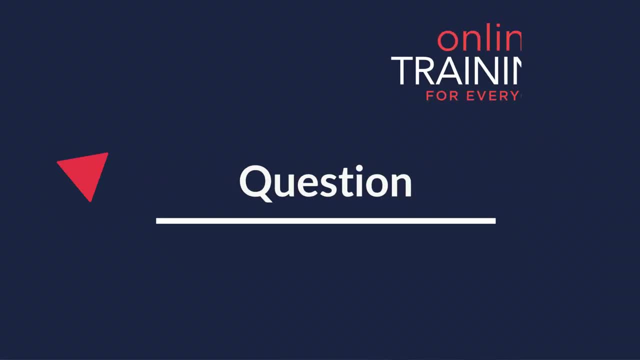 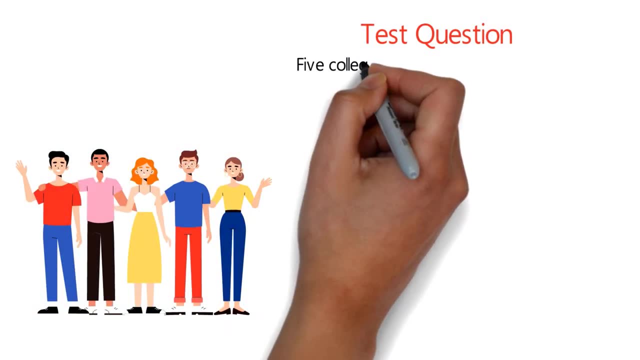 ready for the test. Here's an interesting question you may need to know. Well, not just for the test, but also if you are trying to rent the house. Five college students together rented a house. One of them decided to move out earlier, and now their 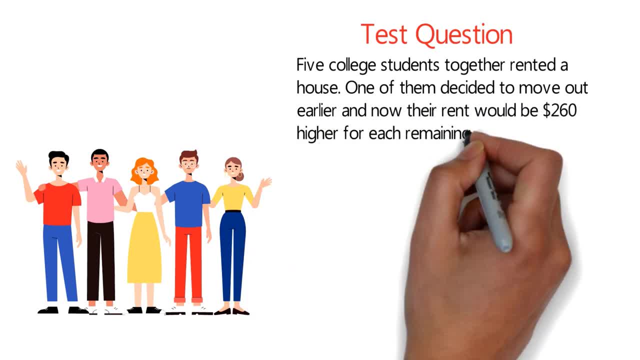 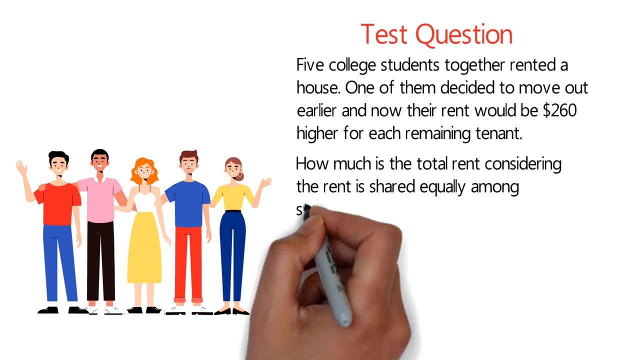 rent would be $260 higher for each remaining tenant. What is the cost of the total rent, considering? the rent is shared equally among students And you are presented with four different choices: Choice A: $5,200.. Choice B: $3,120.. 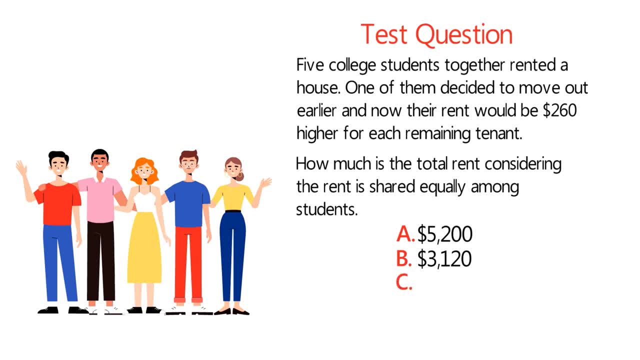 Choice C: $2,600. And Choice D: $2,340.. Give yourself 20 to 30 seconds. maybe pause this video to see if you can come up with the answer on your own. Let's go ahead and solve this challenge together- One of the easiest. 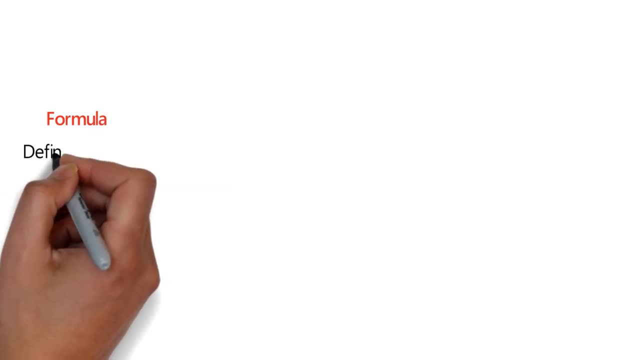 ways to solve this challenge is to create a formula. Let's start by defining a variable. We will define this variable as S, which would represent an initial split rent for five students. So, using this formula, we can calculate the total house rent as five multiplied by S. 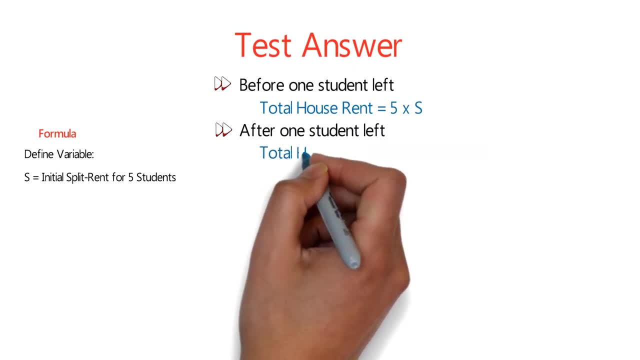 which means that after one student left, the total house rent could also be calculated as four multiplied, and then the value in parenthesis S plus $260.. Using both approaches, we can create an expression: 5 multiplied by S equals 4 multiplied, and then the value in parenthesis S plus $260. 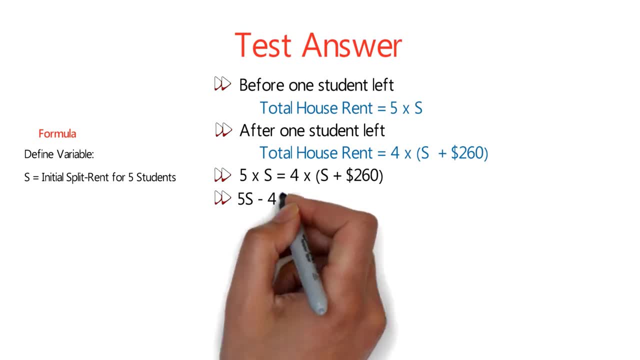 Once we simplify it, we'll get to the equation: 5S minus 4S equals $1,040, which means that the S equals $1,040, which represents initial one student rent. To calculate total house rent, we need to multiply 5 by $1,040.. 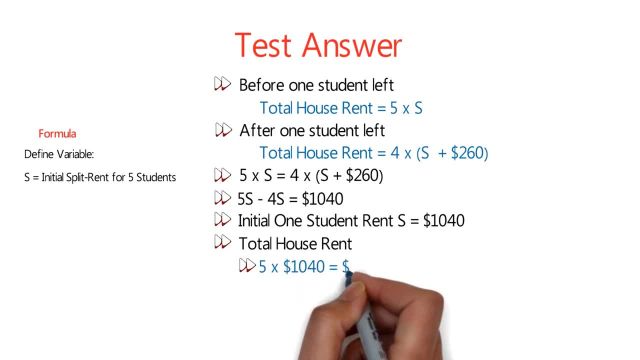 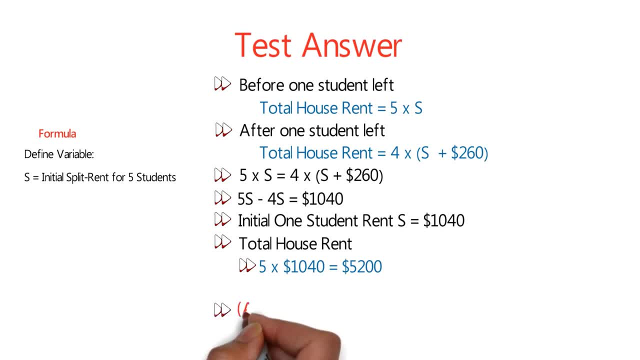 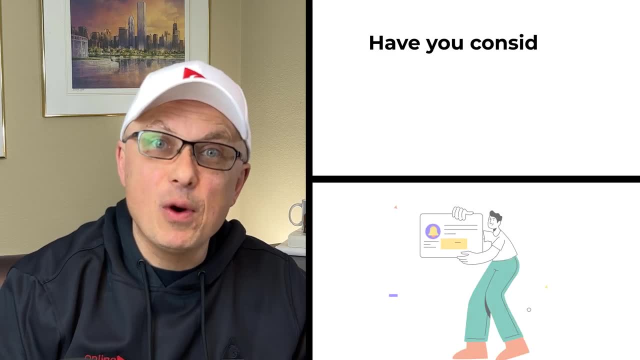 And the result will be $5,200.. So the answer is choice A- $5,200.. Hopefully you've nailed this question and now know how to answer similar questions. I have a question for you: Have you considered subscribing to online training for everyone? 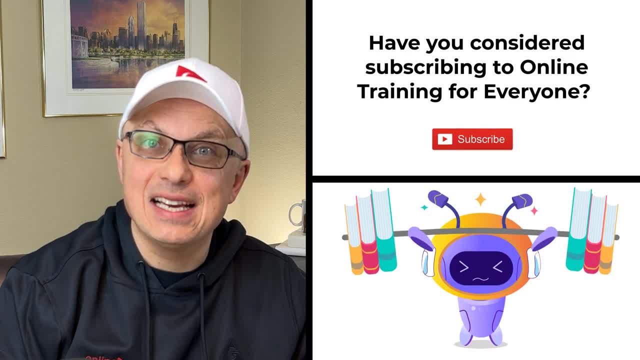 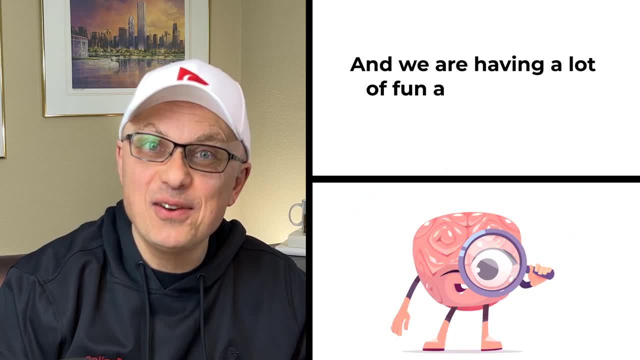 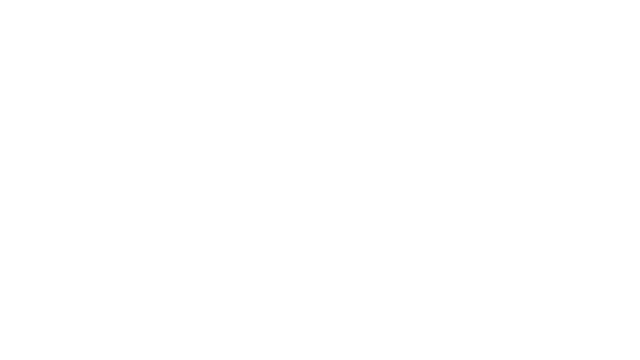 We focus on helping you not just to get ready for assessment test, but using our materials, you can also improve your concentration, IQ and brain power, And we're having a lot of fun along the way in this process. Thank you for considering, and now let's continue and get you ready for the test. 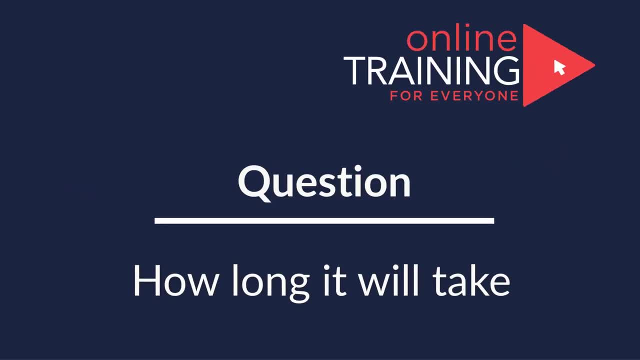 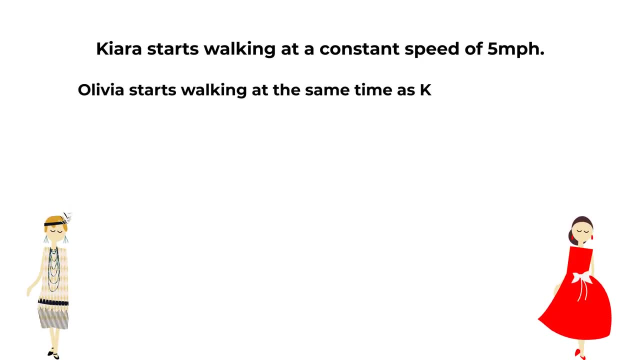 Here's an interesting question we frequently see. on the test, Kiara walks at the constant speed of five miles per hour. Olivia starts walking at the same time as Kiara, but starts four miles behind her and walks at a constant speed of eight miles per hour. 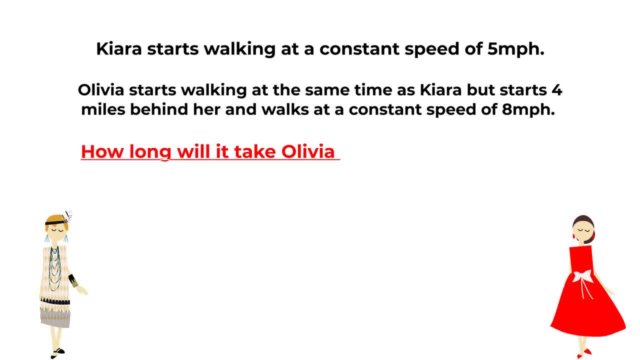 How long will it take for Kiara to catch up with Olivia? You're presented with four different choices: Choice A- 50 minutes, Choice B- 60 minutes, Choice C- 70 minutes And choice D- 80 minutes. 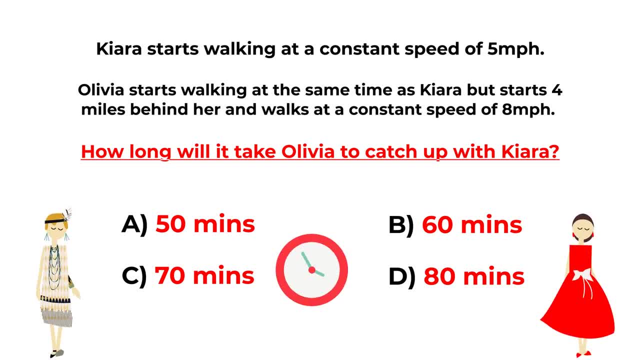 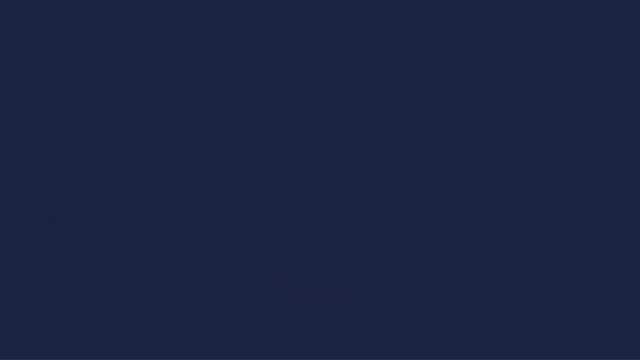 Do you see the answer? Give yourself a little bit of time and think about all possible combinations. Ready or not, let's move forward and get to the correct solution together. One important consideration to help you solve this challenge is that the speed for both. 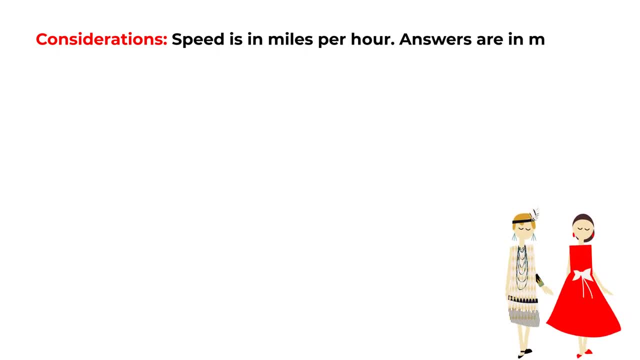 Kiara and Olivia is presented in miles per hour, But answers are easy In minutes, So at some point we would need to make a conversion. Another important point is that both Kiara and Olivia will walk the same time and we can put it as x in hours before catching up, because they started at the same time. 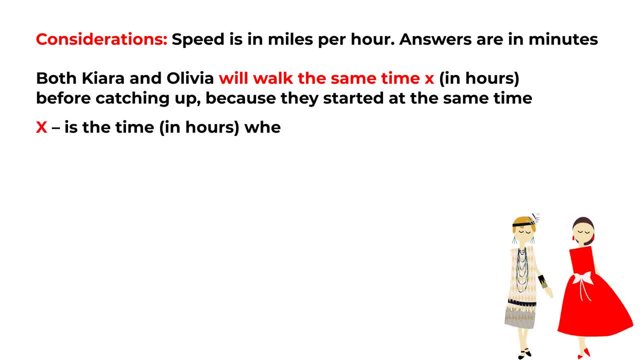 In our solution. x will be the time in hours when they will catch up and meet. To solve this challenge, we need to build an equation: 5x plus 4 equals 8x. 8x represents how much Olivia can walk. 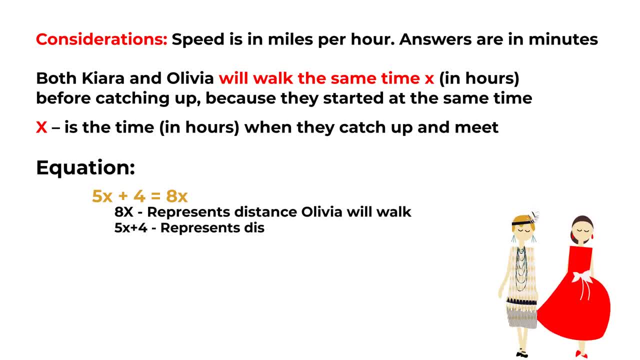 5x plus 4 equals 8x, How much Olivia will walk, And 5x plus 4 is representing how much Kiara can walk, And the starting point for this will be starting point of where Olivia starts, Since Olivia starts 4 miles behind. 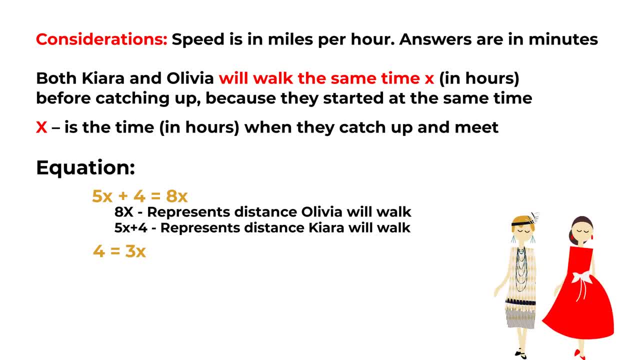 So if we simplify this equation, 4 will be equal to 3x And x will be equal 4 thirds, or 1 and 1 third of an hour. And now is the time to do the conversion. One hour equals 60 minutes. 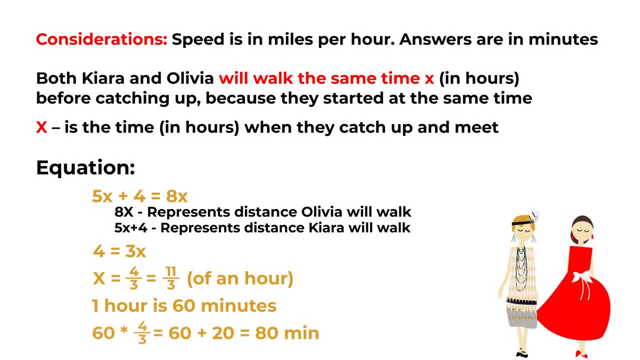 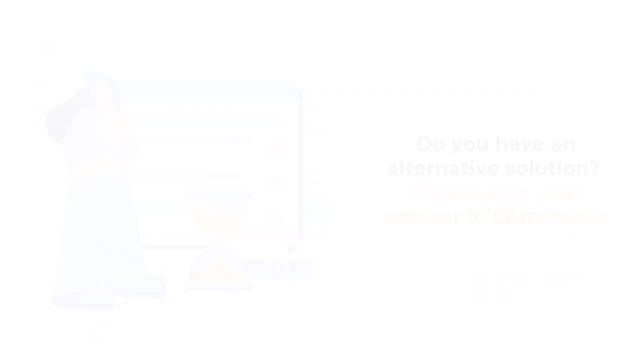 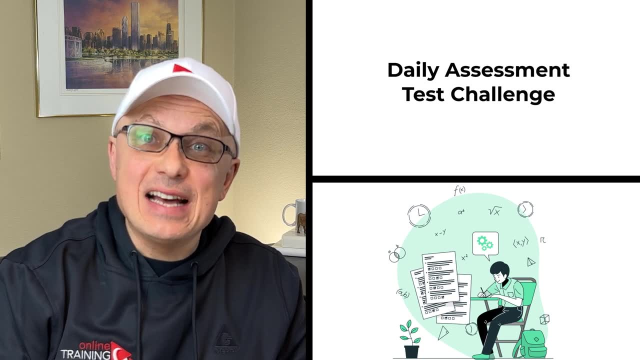 60 multiplied by 4 thirds equals 60 plus 20 equals 80 minutes. So the correct answer here is choice D, 80 minutes. Hopefully you've nailed this question and now know how to answer similar problems on the test. I would like to ask you to participate in our daily assessment test challenge. 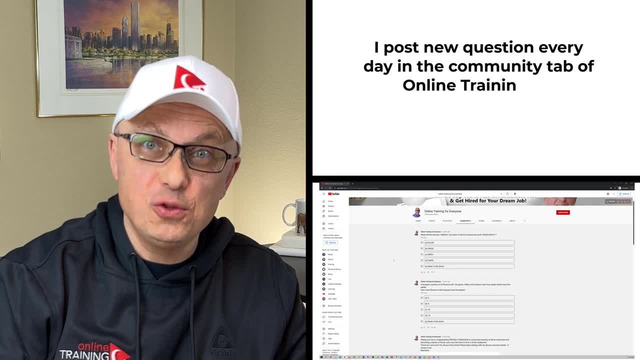 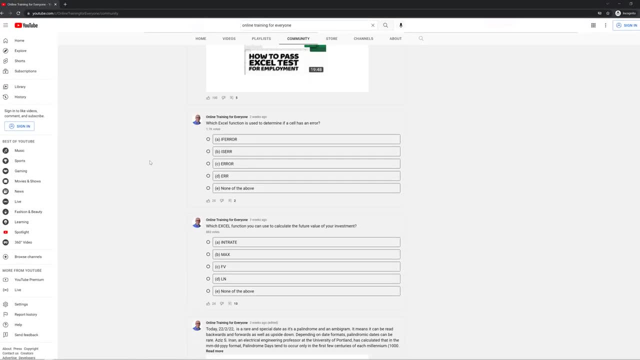 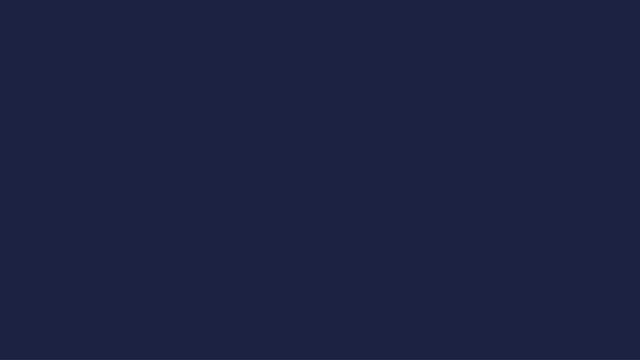 I post new question every day in the community tab of YouTube channel and give you an opportunity to answer it and try it, And I post answer in comments next day. So please make sure to check it out, to test your knowledge. And now let's continue and get you ready for the test. 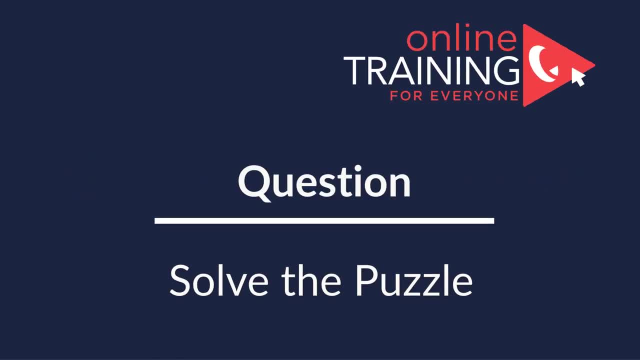 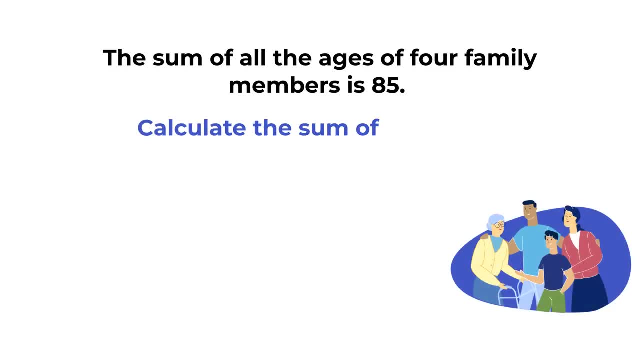 Here is the puzzling question that you might frequently see on the test, The sum of all the ages of 4 family members is 85. What would be the sum of their ages together in 5 years? And you are presented with 4 different choices. 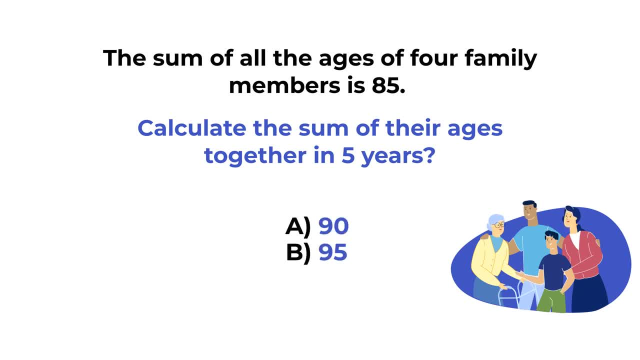 Choice A: 90.. Choice B: 95.. Choice C: 100.. And Choice D: 105.. Do you see the answer? Give yourself 20 to 30 seconds to see if you can come up with the solution, Ready or not. I am moving forward to get to the correct solution together. 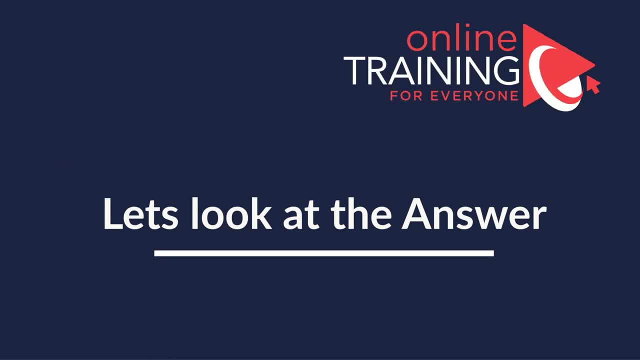 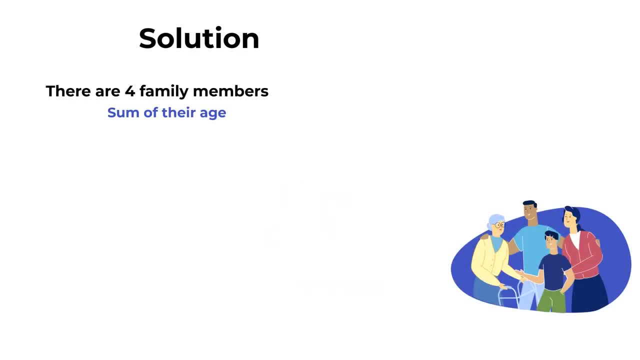 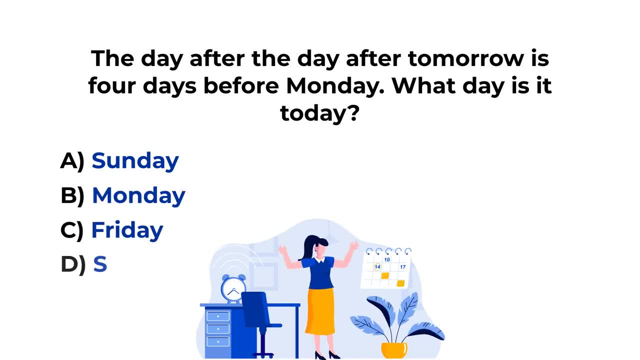 And in 5 years they are 85.. Feel free to Pause this video to see if you can come up with the solution. I would like to give you a hint. The best way to solve this type of problems is using reverse calculations. 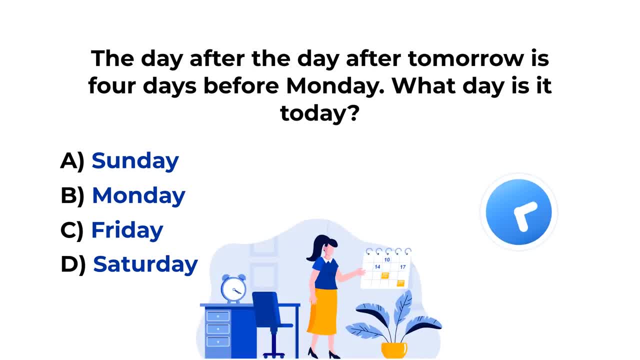 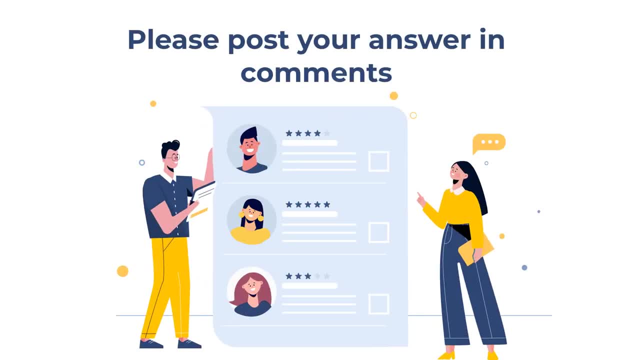 So do you see the answer? Give yourself 10 to 15 seconds to see if you can come up with the solution. Did you figure out the answer? Make sure to post your answer, as well as your rationale for solving this problem, in the comments section of this video. 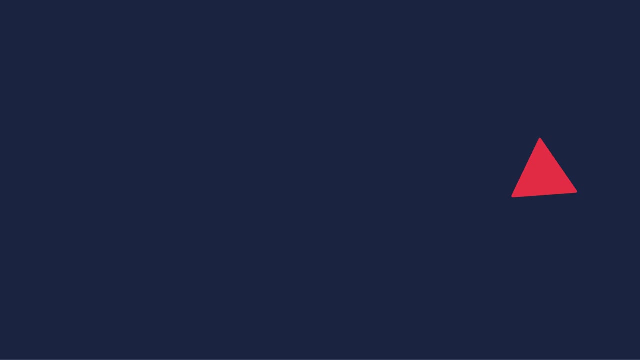 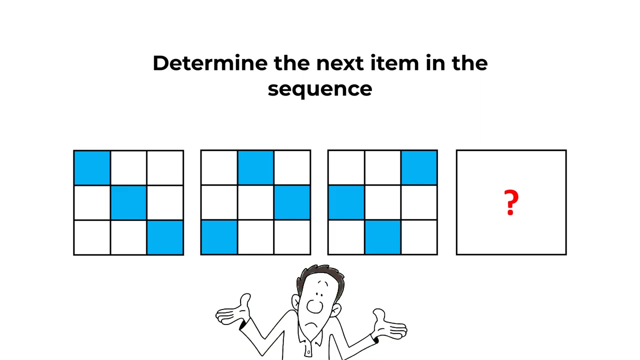 Thanks for participating and good luck. Here is a very interesting problem that you might frequently get on a test. You need to determine the next item in the sequence. You are presented with the sequence of large squares. Each large square contains nine small squares inside. 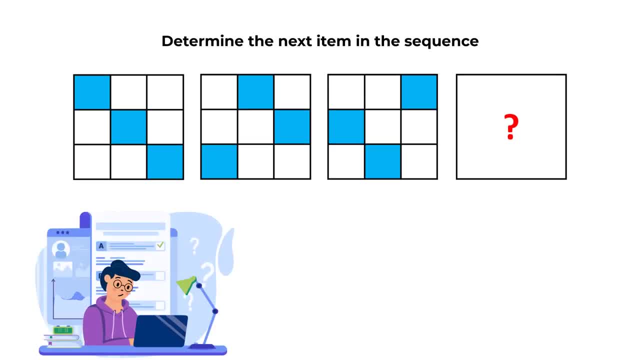 And small squares are of the different color. You need to determine next item in the sequence And you have four different choices: Choices A, B, C and D. Do you see the answer? Give yourself 10 to 15 seconds. 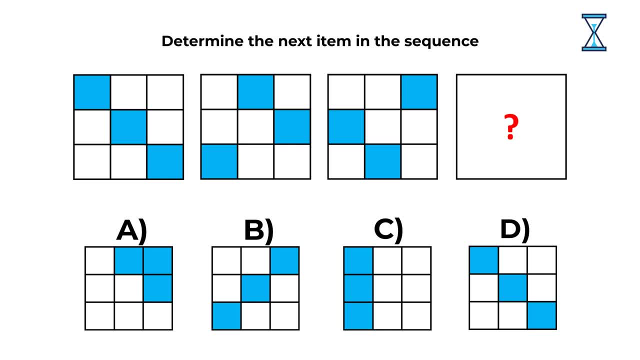 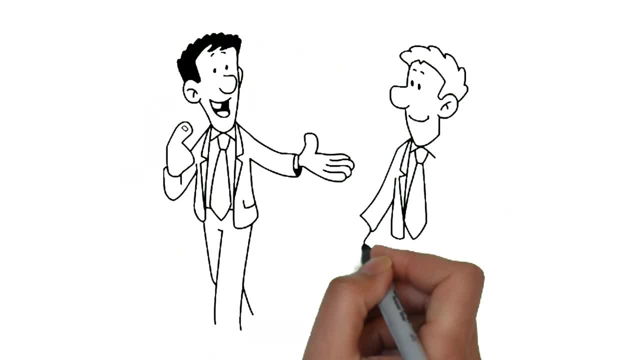 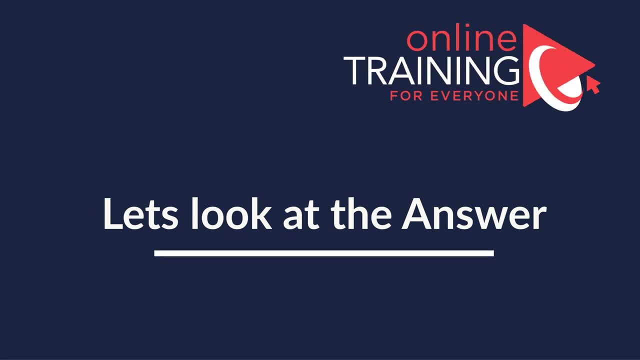 Maybe longer, Maybe 20 to 30 seconds, to see if you can come up with the solution. Did you figure it out? Let's go ahead, move forward to get to the correct solution together. As always, my advice to you: look for patterns. 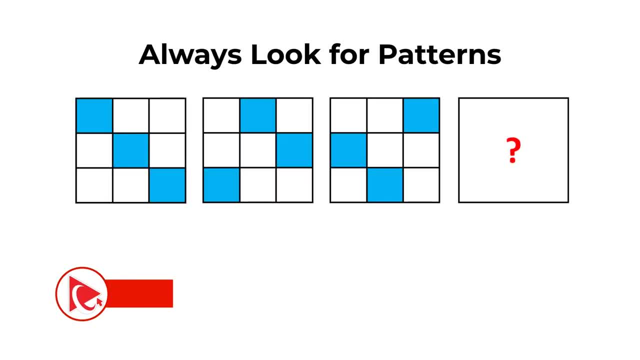 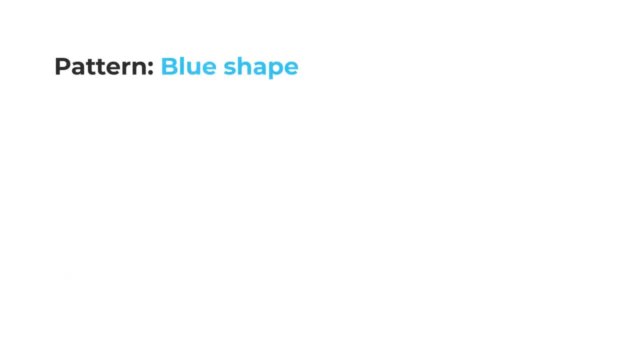 And determining the pattern is key to solving this particular problem. What you need to know to answer this particular question is that blue shape moves within the row of the larger shape. In each row, blue shape moves from left to right one step at a time. 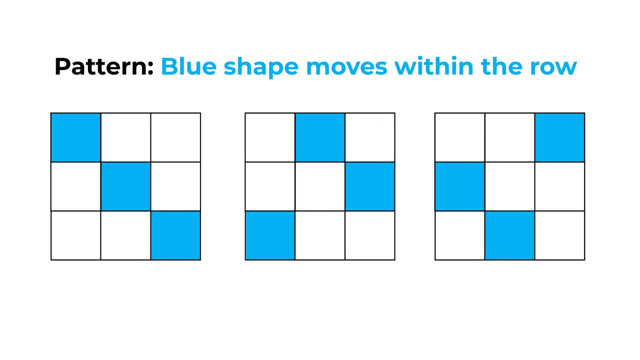 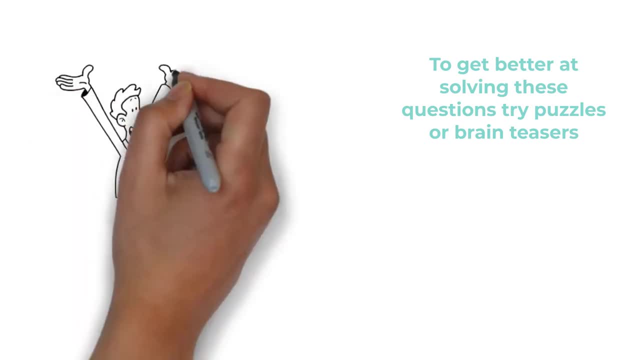 And once blue shape reaches the end of the row on the right, it reappears on the left. So the correct answer here is choice D. Hopefully you've nailed this question and now know how to answer similar problems on the test. Can I ask you to do me a favor? 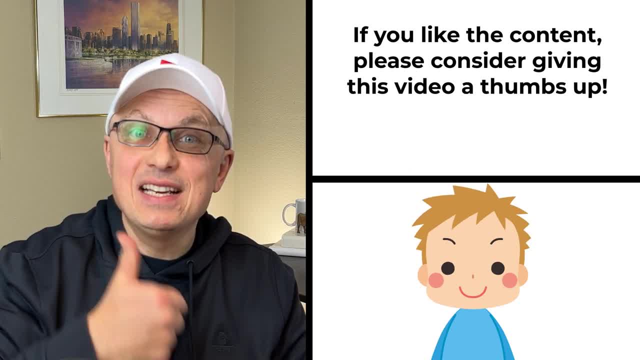 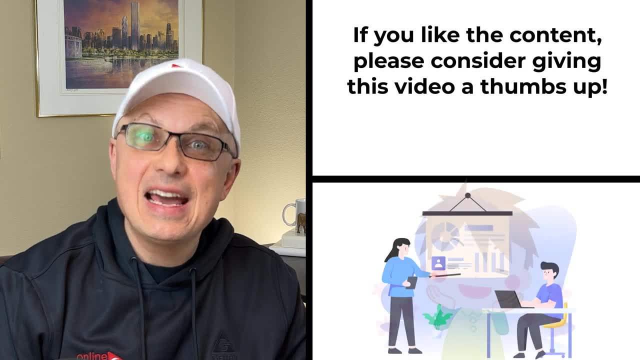 If you like this content, can you please give this video big thumbs up? This tells us that you need more content like this, and we'll make sure you will get it in the future. And now let's continue and get you ready for the test. 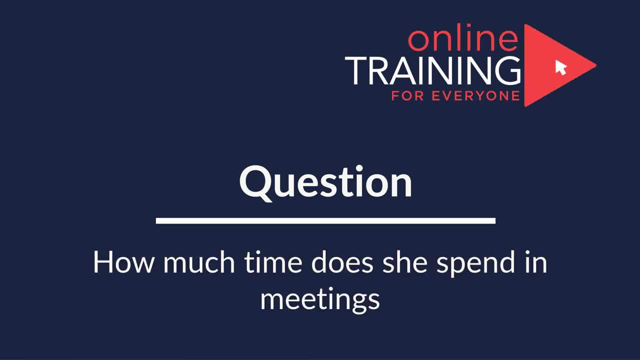 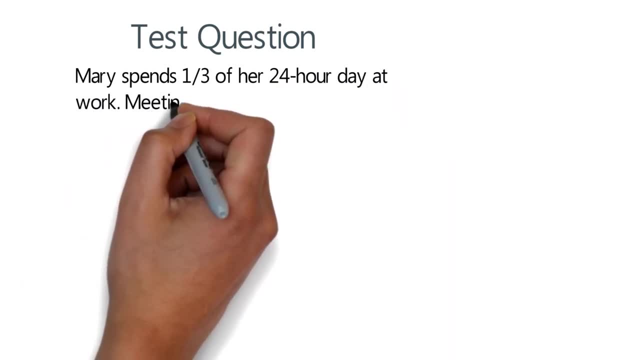 Here's an interesting question which validates how well you do planning of your day-to-day work. Mary spends one third of her 24-hour day at work. Meetings take one fourth of her workday. How many hours does she spend in meetings? 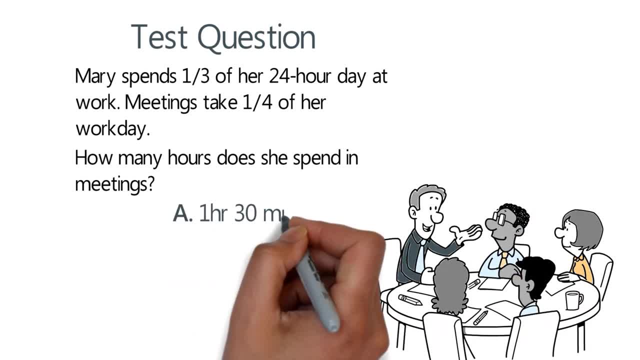 You have four different choices: Choice A- one hour and 30 minutes. Choice B- two hours. Choice C- two hours and 30 minutes. And choice D- three hours. Give yourself 10 to 15 seconds, maybe a bit longer. 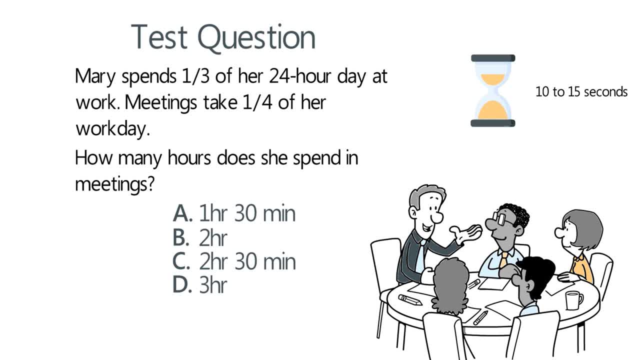 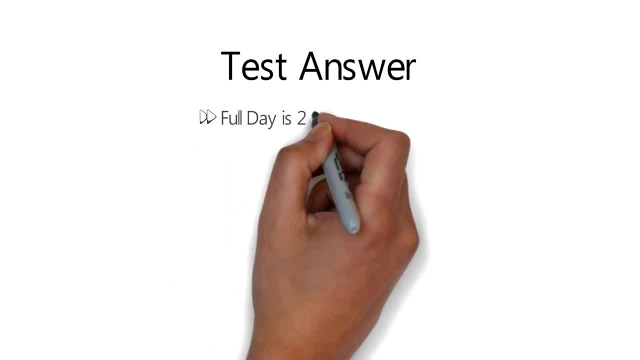 depending how well you typically solve these types of problems. Ready or not, let's go ahead and solve this challenge together. As you might be well aware, full day has 24 hours. Mary's working hours are very typical. They represent one third of the full day, which is eight hours. 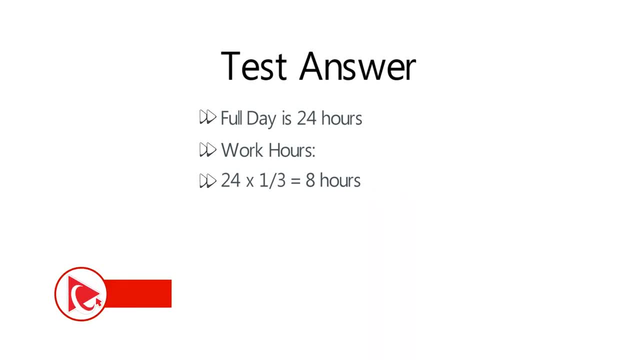 And we calculate it by multiplying 24 by one third, or actually dividing 24 by three. Meetings take one fourth of her workday. So to calculate how much time she spends in meetings we need to multiply eight hours by one third of the full day. 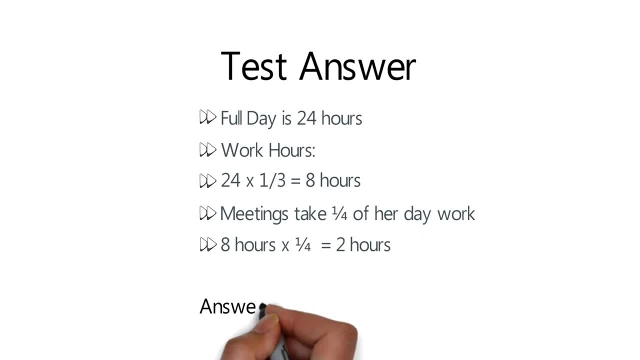 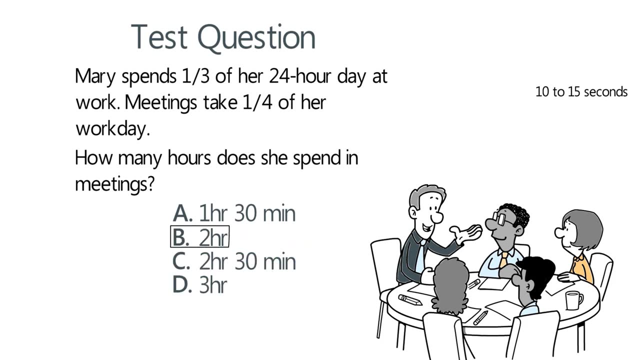 So we have one fourth And the result is two hours. So the correct answer is choice B, two hours. Hopefully you've nailed this question and now know how to answer similar problems in the test. One of the most frequent questions I get is to provide the best techniques. 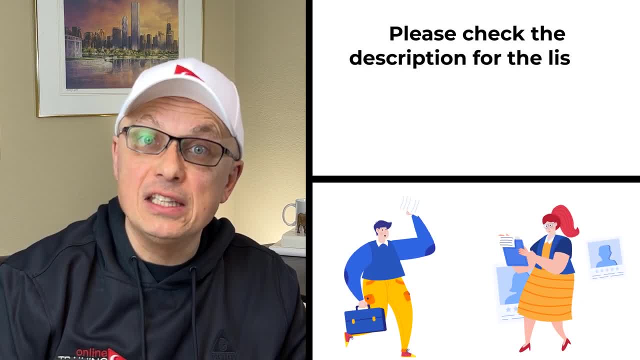 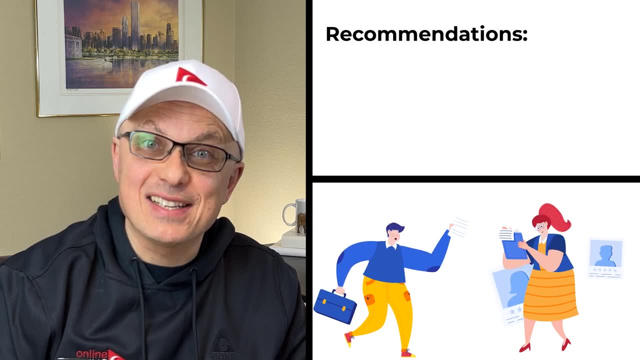 to get prepared and pass the test. We put together a list of resources that might be helpful for you in the description section of this video. Obviously, taking sample tests and reviewing questions and answers is a must, But some list of resources that might be helpful for you in the description section of this video. Obviously, taking sample tests and reviewing questions and answers is a must. 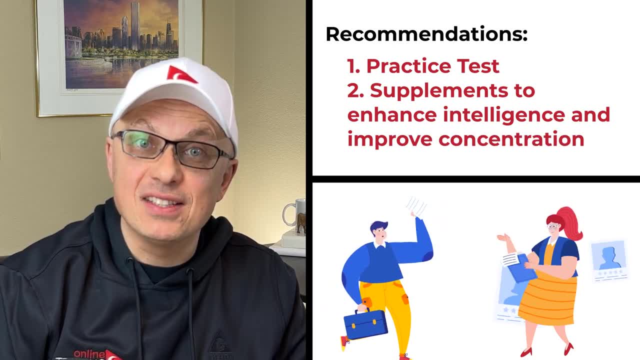 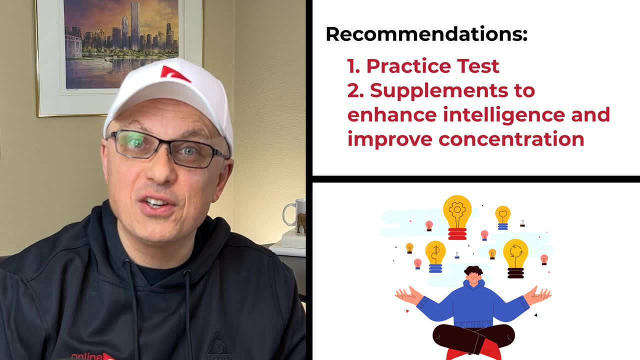 But some list of resources that might be helpful for you in the description section of this video. Sign up for free trials with educational training vendors and even use special supplements to improve your brain function and concentration. I put links to our trusted partners for the products I use. 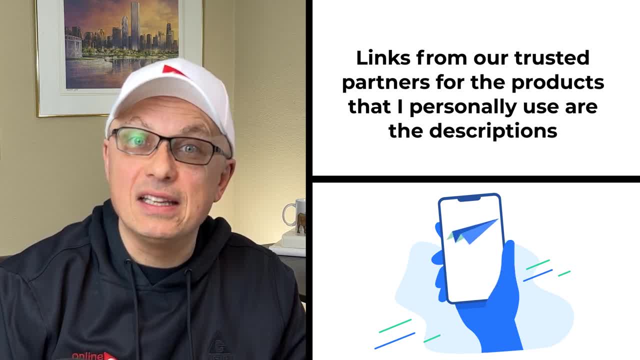 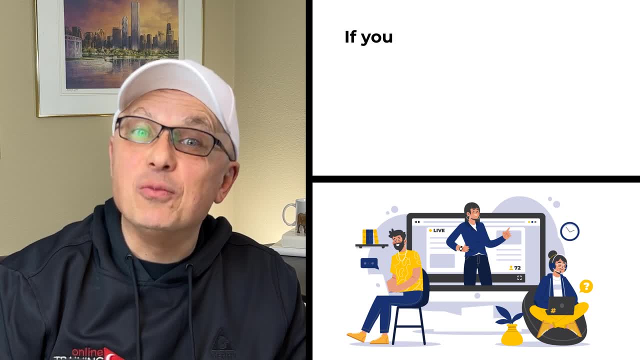 in the description section of this video. Some links might be affiliate, which means that I will get paid a small fee without increasing costs to you. Make sure to check them out. And one request for you, If you know any other helpful resources: 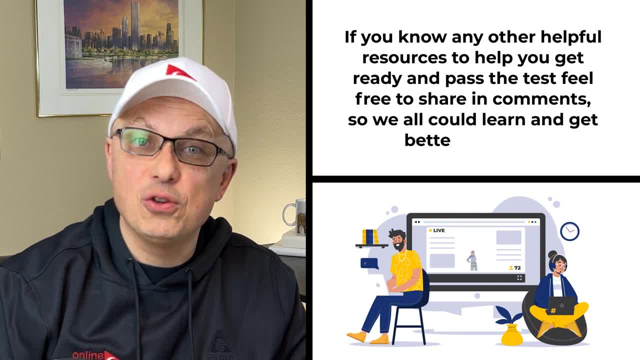 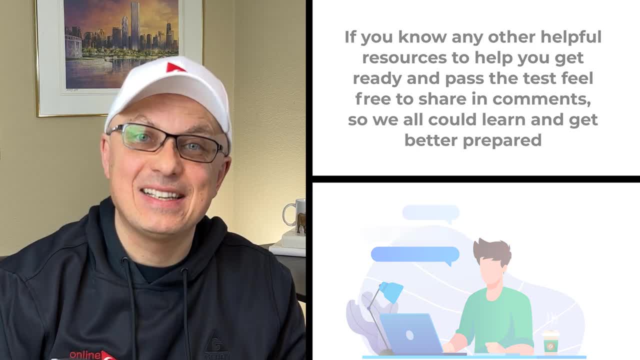 resource to help you get ready and pass the test. feel free to share it in comments so we could all learn and get better prepared. And now let's continue and get you ready for the test. Here's the interesting question, which is easy to understand, but at the same time, you will have a. 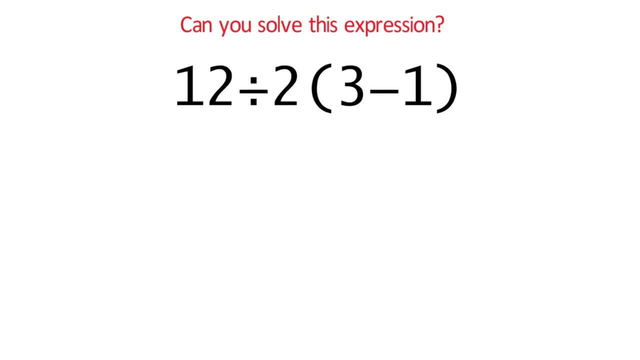 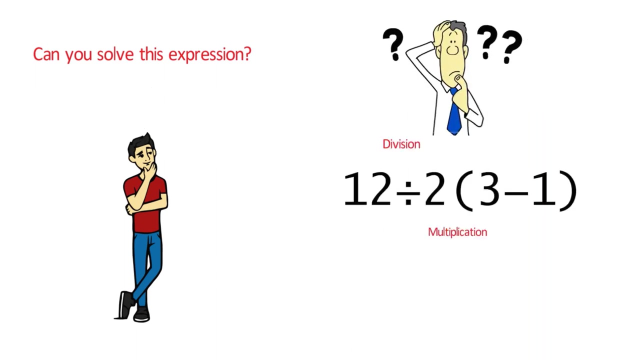 lot of fun solving it. You need to calculate the simple expression 12 divided by 2 and then multiply it on the value in parentheses, which is 3 minus 1.. Take a look closely and see if you can come up with the answer. There are three operations here: division, multiplication and 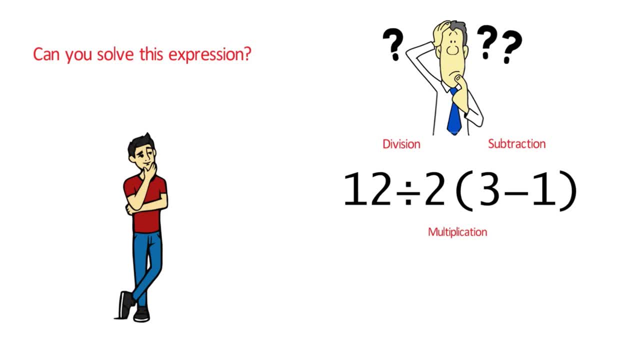 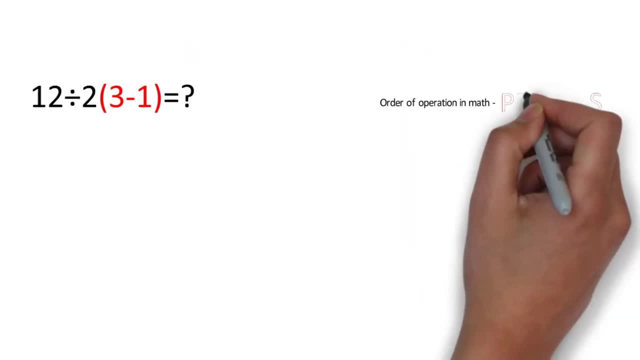 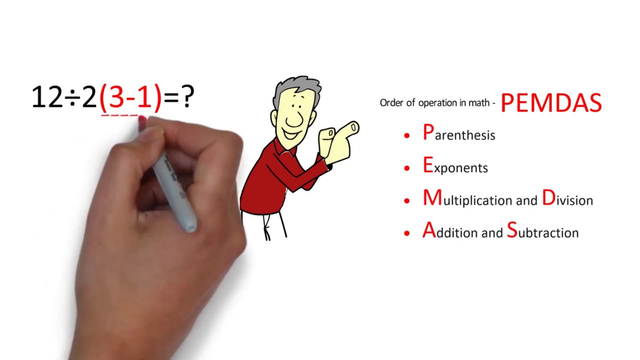 subtraction. All you need to determine is which one to do: first, second and third. Do you think you know the answer? Let's continue and get it solved together. The order of operations in math tells us that the first expression we need to solve is in parentheses. We first need to calculate. 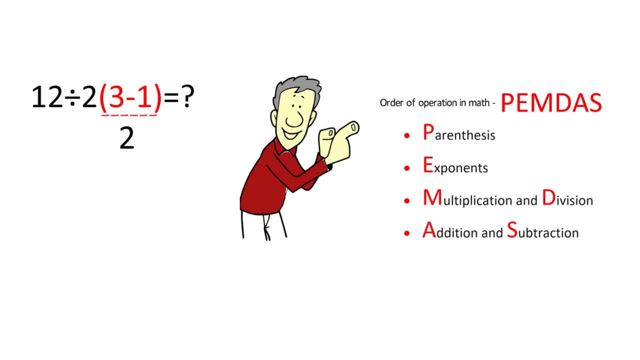 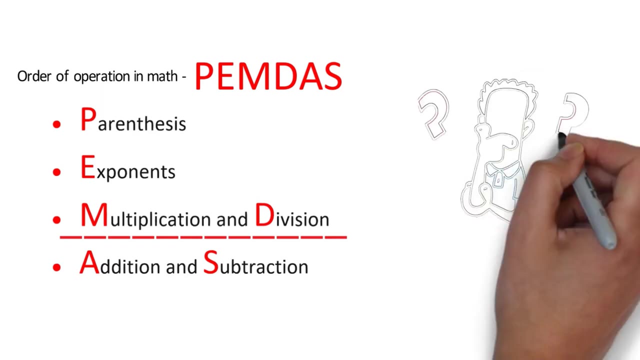 3 minus 1.. And obviously the answer is 2.. The big question is: what do we do next? The order PEMDAS tells us that we need to do multiplication and division, But what order doesn't mention is that we need to do it from left to right. 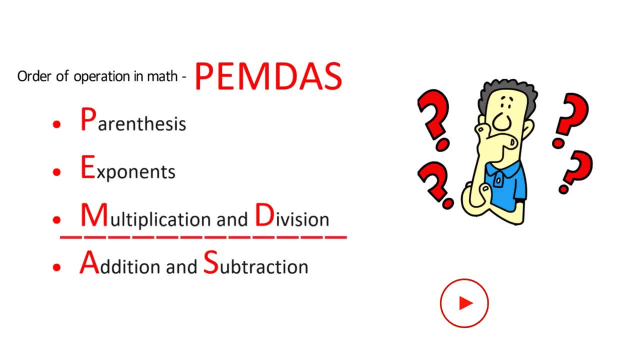 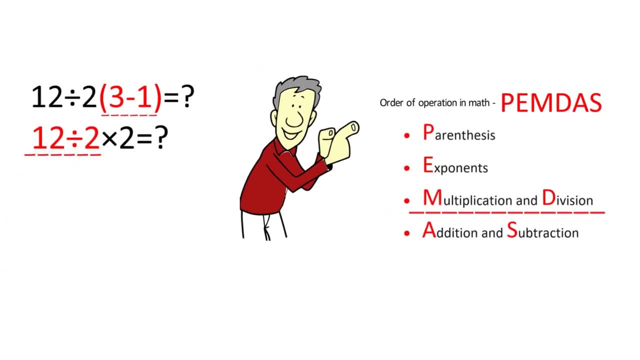 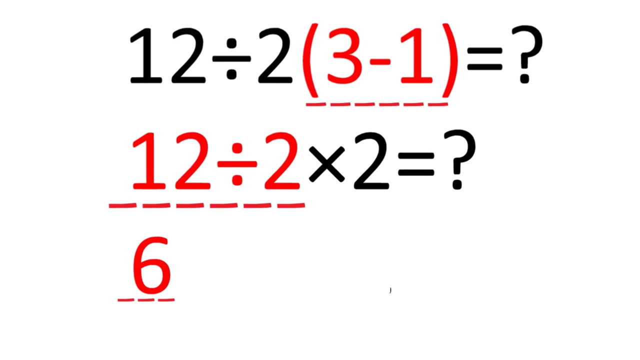 And, what's interesting, the acronym itself is a little bit confusing because it shows multiplication first and then division. But in our case we need to do division first and divide 12 by 2 and then do multiplication. Once we divide 12 by 2, we get to 6 and the 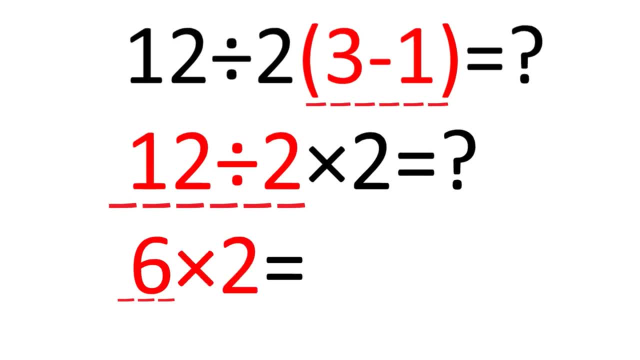 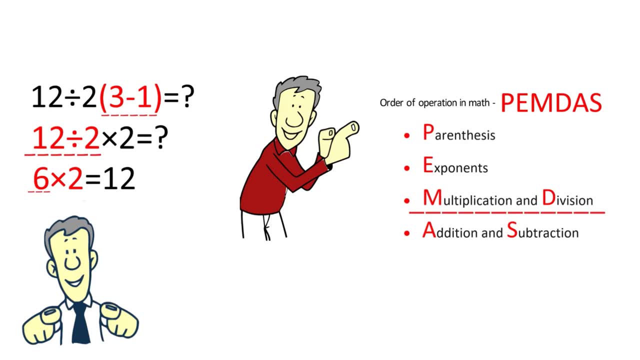 final expression we need to solve would be 6 multiplied by 2.. So the correct answer here is 12.. So did you solve this challenge on your own? Was it easy for you? Please share your thought process and your solution in the comment section of this video. Here's the cool question.